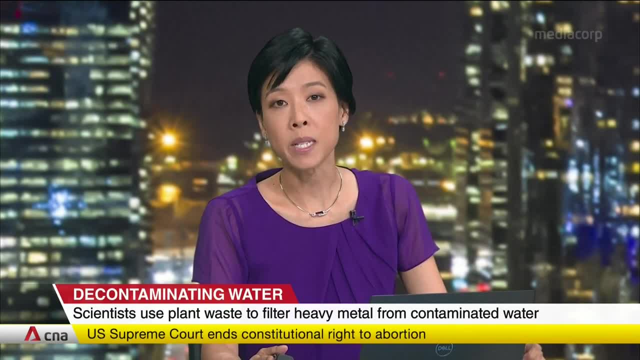 to make peanut and sunflower oil. Research team from Singapore's NTU and ETH Zurich in Switzerland says that protein membranes can filter out heavy metal in contaminated water. For this, Professor Ali Mizawe from NTU, who is the principal investigator of this research, 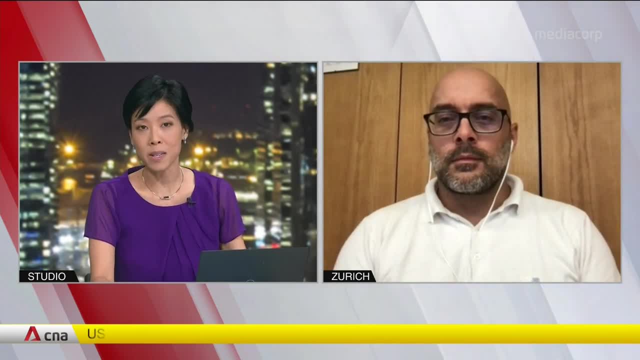 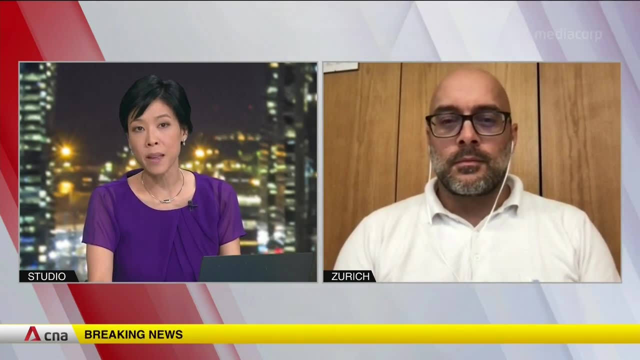 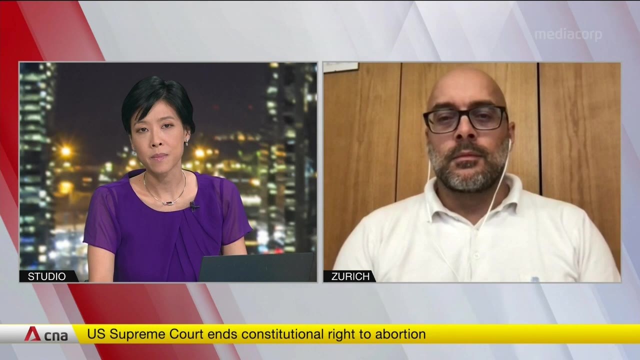 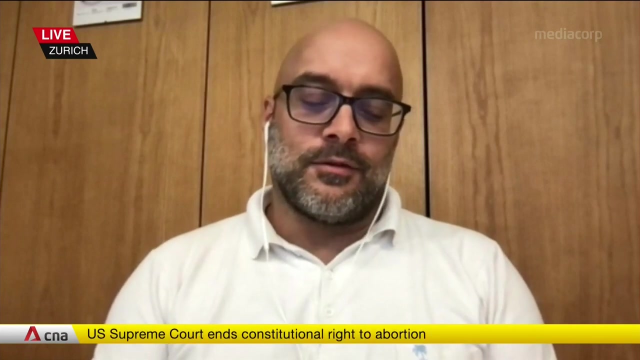 joins us. Professor, I think I just outlined how this works. Essentially, it's using these waste products, combining them with activated carbon to produce a membrane that attracts, and therefore filters off, these heavy metals. Is that how this works? That's absolutely correct. You understood it very well, And so, to give a bit more, 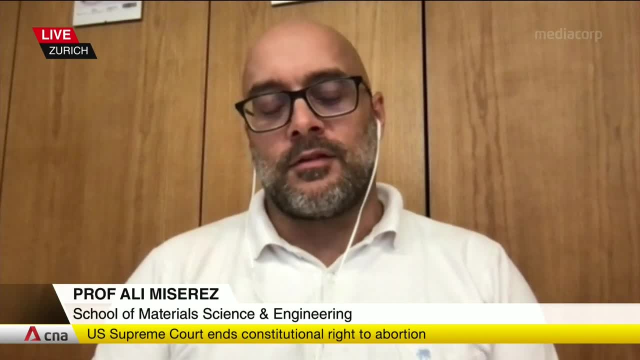 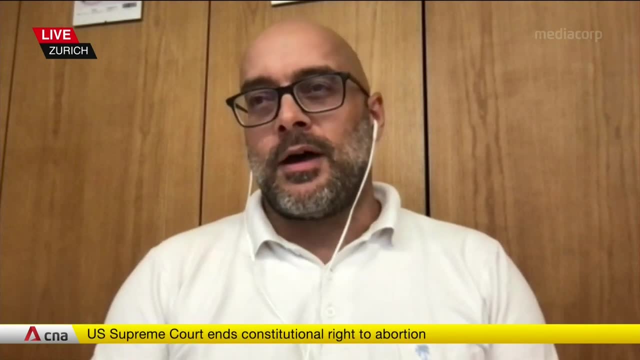 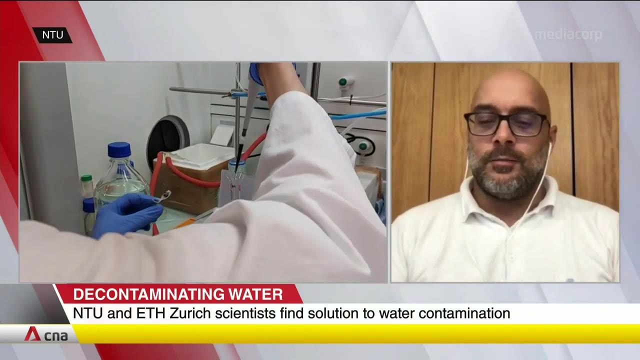 detail. basically, you can think about those filters as molecular sponge. So we take those proteins, we can make some very small fibers that are about 10 times smaller than human hair And then, when you filter the water through, it will absorb the heavy metal contaminants. 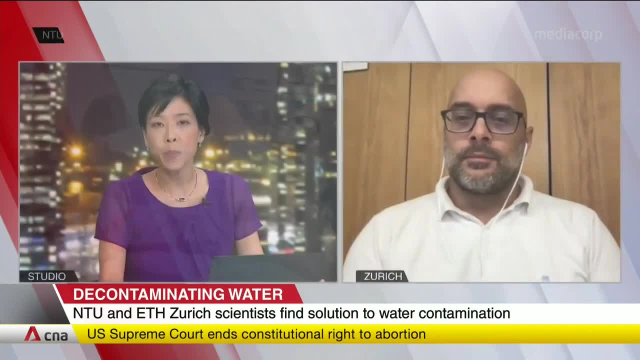 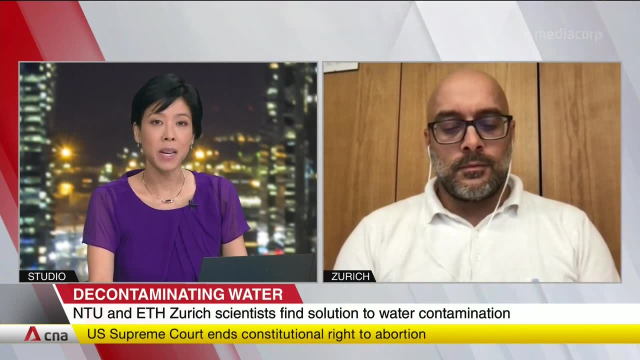 Oh, one of the huge benefits of should you make it something that's scalable is that it's cheap. it does not require any kind of power to run, and therefore you can use this in countries where the issue is, for example, 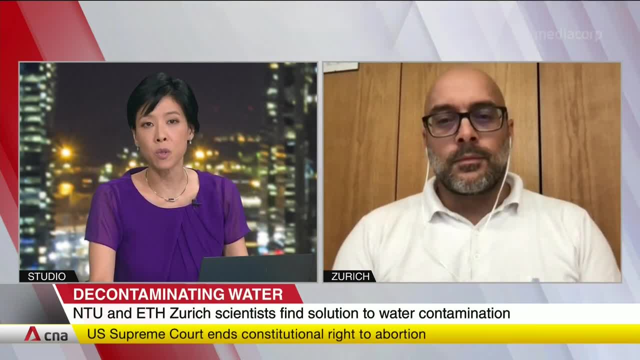 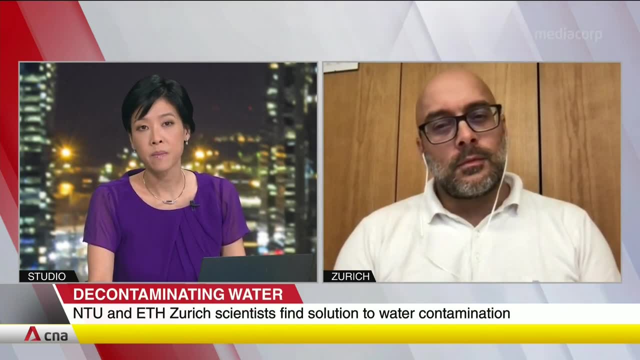 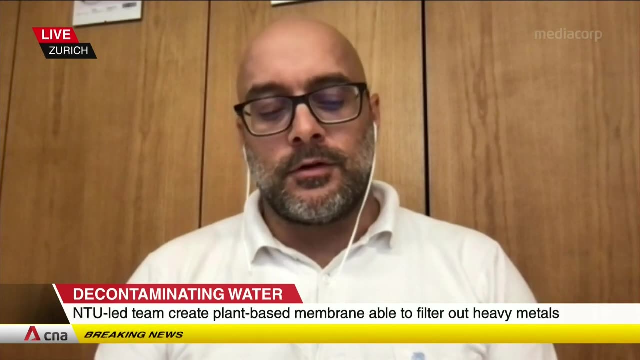 with electricity. What other advantages are there to using this protein to combine it and then use it to filter off heavy metals? So one of the advantages is it is a universal, so you can filter not only heavy metal but also organic contaminants or even bacteria, That's. 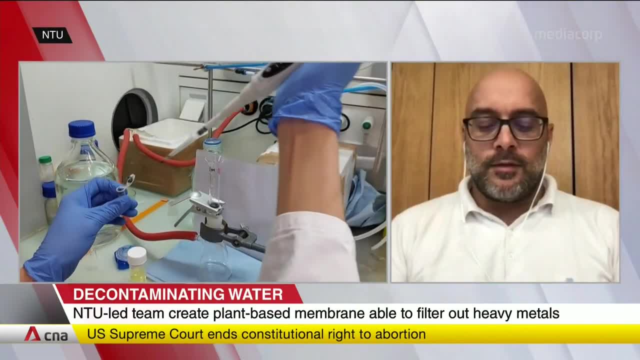 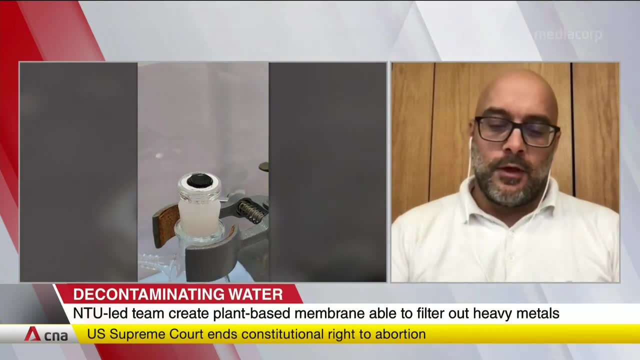 one of the advantages, And then the other one is that, because you have no energy inputs, it's a more sustainable process, because you know when you do water filtration it tends to use a lot of electricity and therefore it's responsible for a lot of CO2 emission. 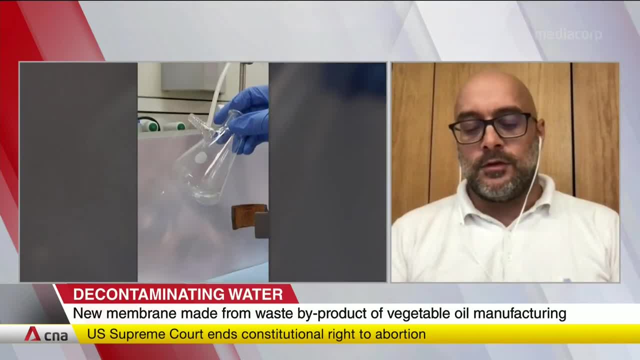 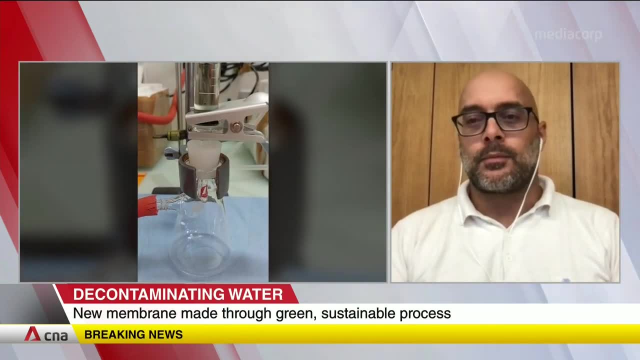 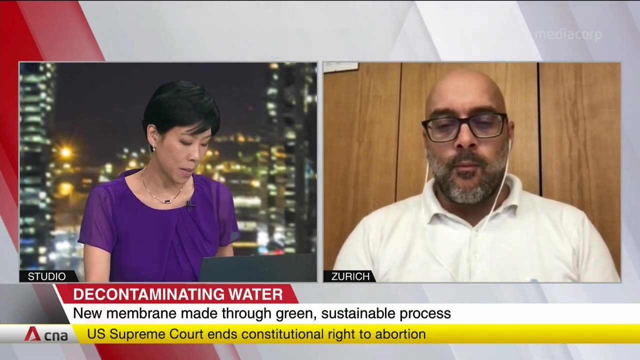 But with this technology, because you don't use any electricity, you can drastically reduce CO2 emission. So that's another advantage of this approach. When we talk about it being scalable and this, you have to make this more clear to a layman like 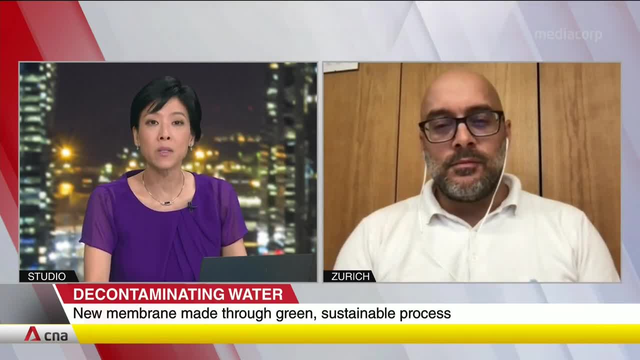 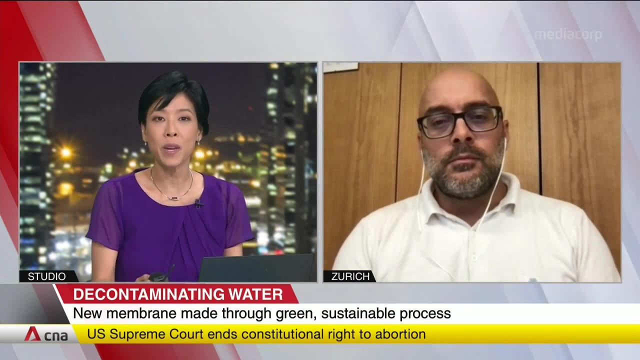 myself. one kilogram of oil seed meal produces 160 grams of protein. So we're looking at really using waste material from, say, a factory that produces peanut oil. How much oil do we need to make, How much waste product from this before we can have a sustainable product? So that's another. 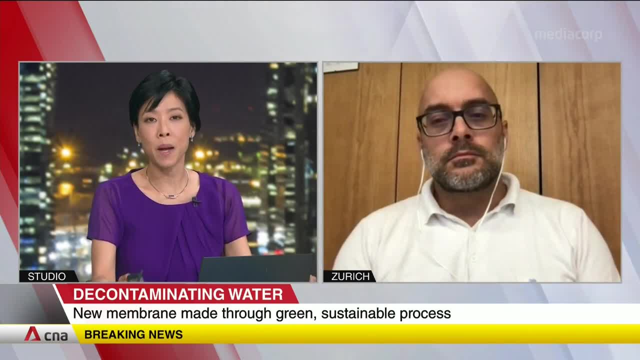 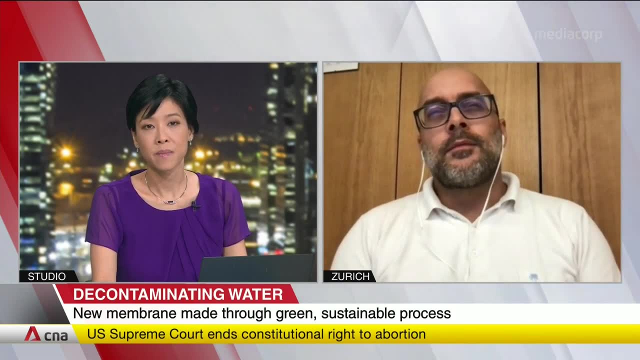 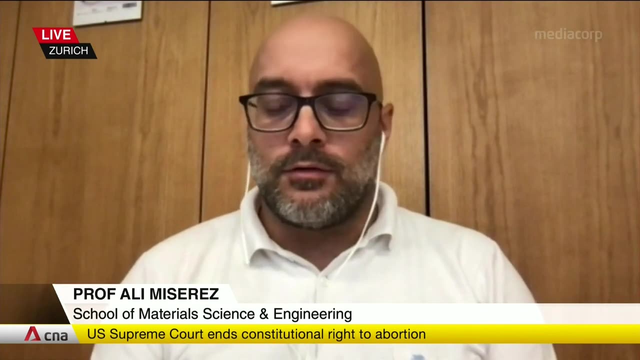 advantage of this approach: sustainable and cost effective water treatment plant that removes heavy metals. So I don't have the exact number in my head, but what I can tell you is that when you produce this kind of oil, you have a lot of those proteins that are just waste, that are unused or they may be. 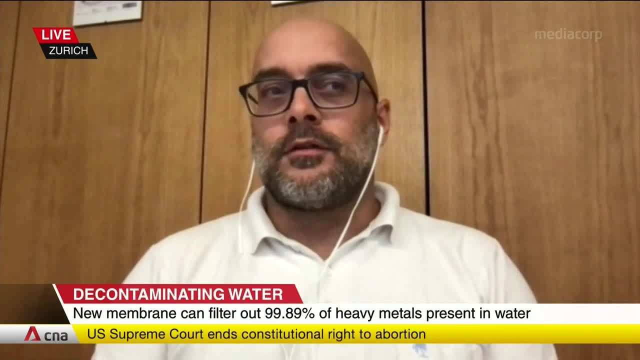 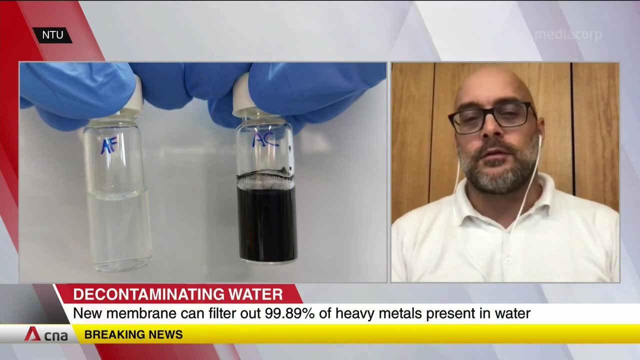 used, given to livestock. So the scale up because it's waste product and a lot of it is generated during production. of those oil you actually have quite a bit available. So the scaling compared to some other technology is actually, I would say, fairly straightforward. 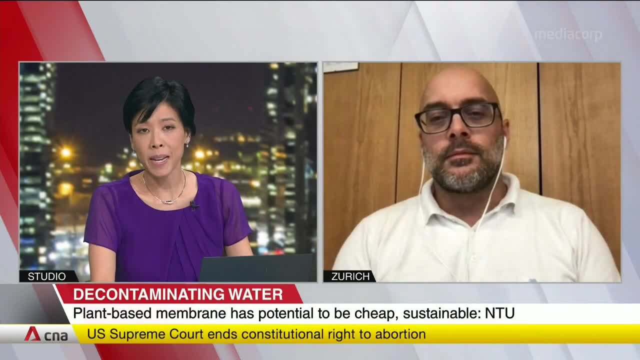 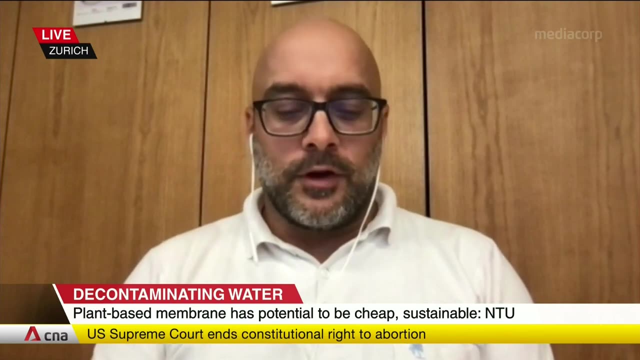 You use the byproducts of peanut and sunflower oil. Can other plant-based materials also be used for this kind of procedure? That's one of the beauty of this technology. You could use any other kind of waste product, but it's not just the byproducts that are used. I mean you could use oil from the plant and you could use. 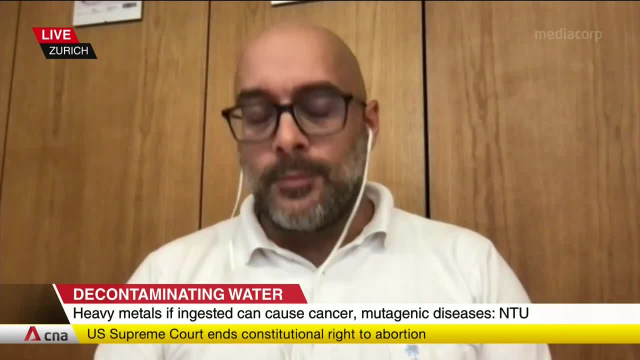 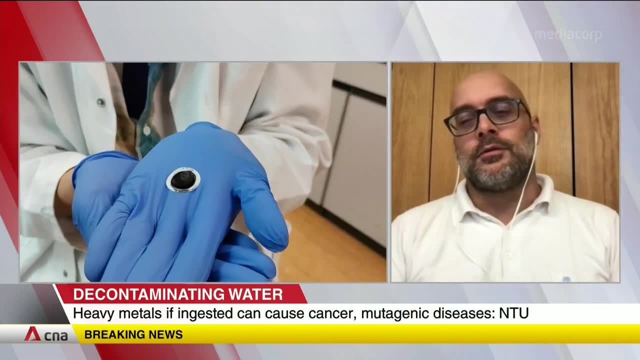 a sizeable gas container. it could be energy, it could be a protein, it could be a soil cereals. You could imagine waste from palm oil production, which is obviously very abundant in Southeast Asia- And those are other options that we could explore in the near future. 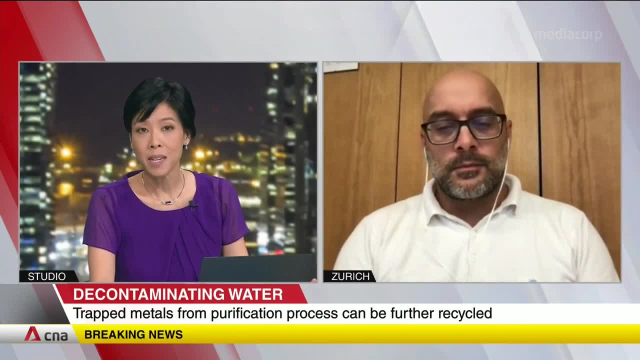 All right, it's in the research stage right now. When, how long do you think you will need before we will be able to see this being used commercially at scale? Yes, Right, That's a good question. I guess it's a quick and simple question. 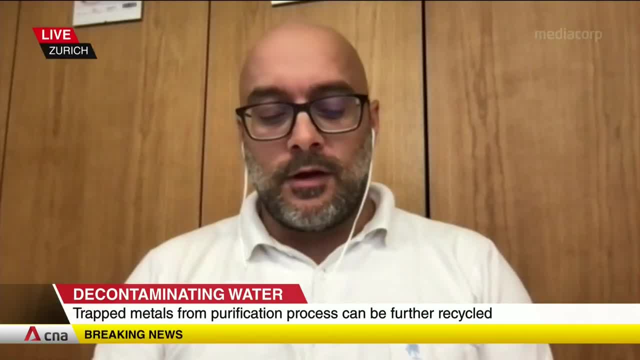 Good, Let's have a look. All right, I have known about you for a long time. Let me give you the name of the company. How do you think your company is? I don't know where to start with you, So it's a bit more advanced, actually, because there's already a spin-off company from ETH Zurich- it's called Blue Act, that we are working with. 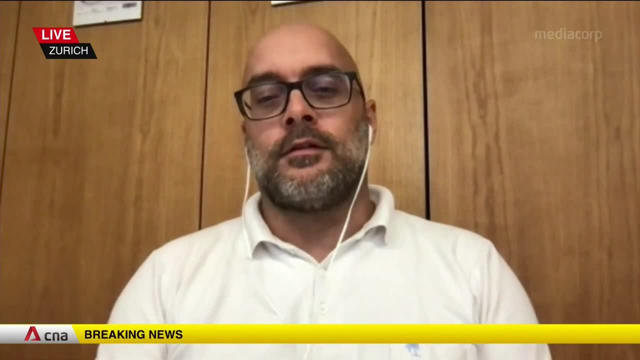 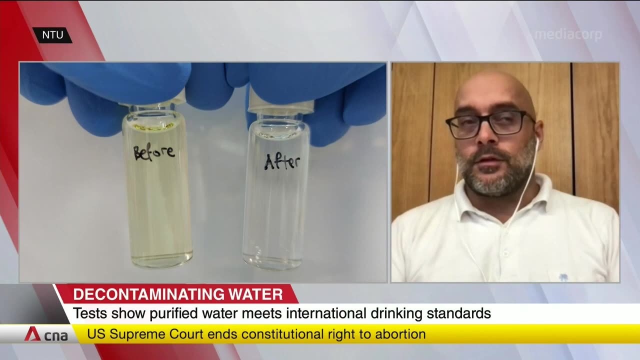 So they have an exclusive license and they're already selling this technology. In fact, it's been used in some pilot plants in Peru, in Sri Lanka and India quite successfully, And we're looking into importing this technology for the Southeast Asian market as well.